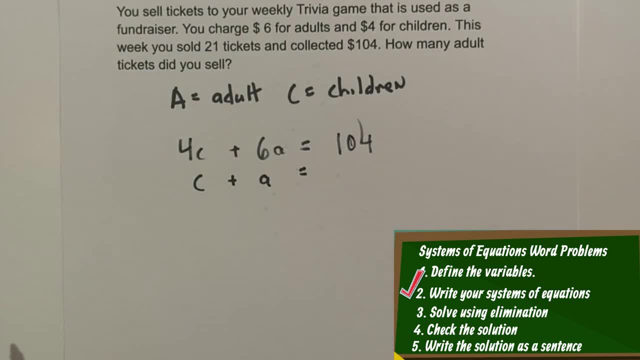 adult tickets, And that equals a grand total of 21.. So we've defined our variables, we've set up our systems of equations. Now we need to use elimination to get down to one variable. So what I can do is: I want 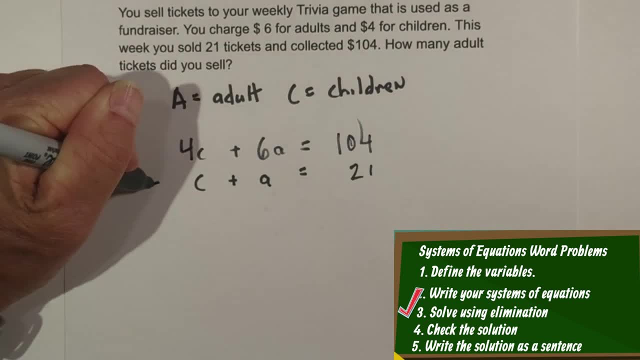 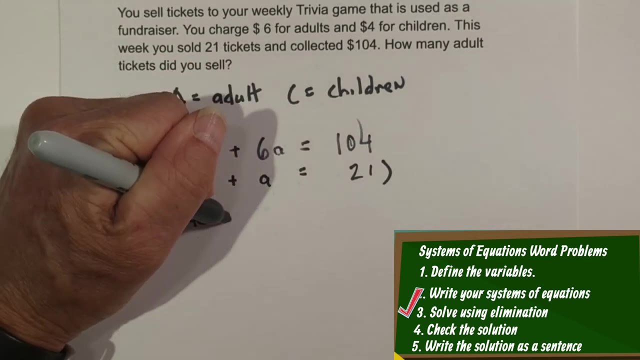 to eliminate the c, so I can multiply all of this by negative four. Okay, And so when I do that, negative four times c is negative four c, And then negative four times 4,, excuse me, negative 4 times a is negative 4a. 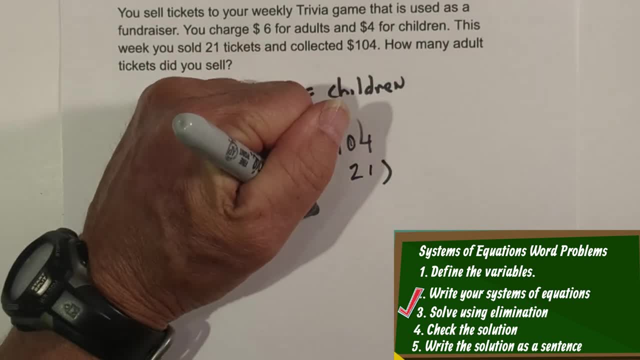 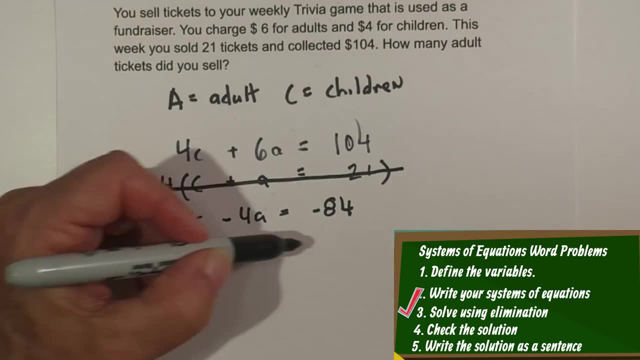 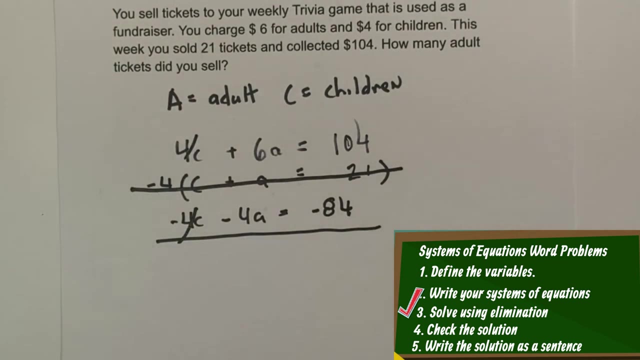 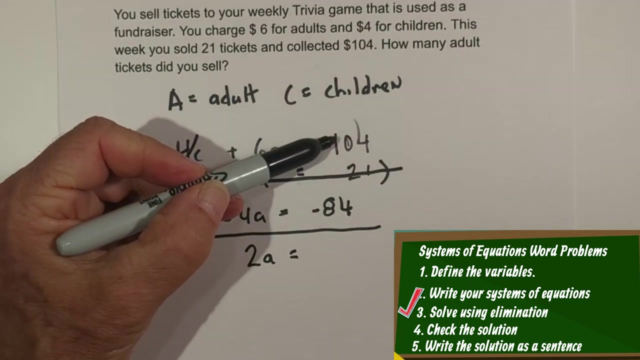 And then negative 4 times 21 is a negative 84,. okay, I'm going to cross this out because I don't like to rewrite a lot, because that's where I make mistakes, So now these cancel, okay. Okay, 6a minus 4a is 2a, equals 104 minus 84 is 20.. 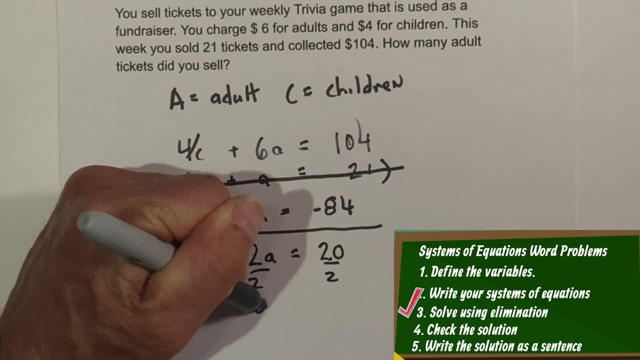 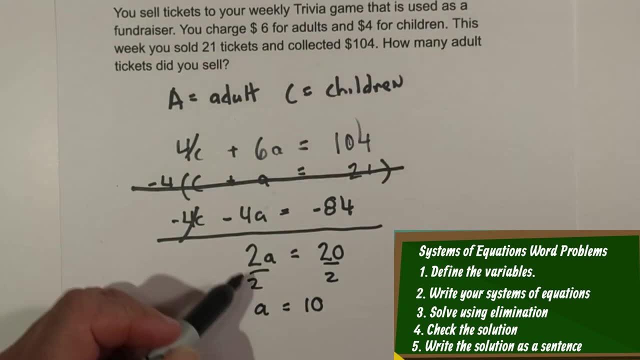 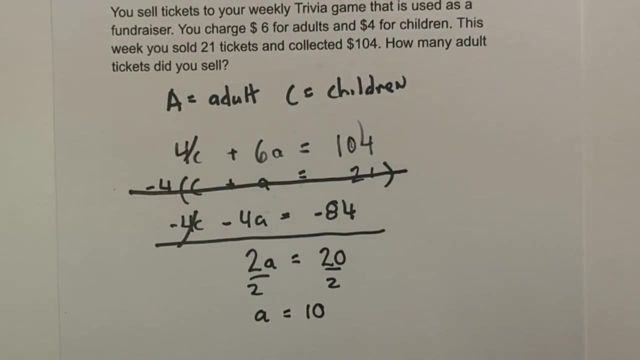 And then I can divide both sides by 2a is equal to 10.. Now, what does that tell us? That tells us that for a, which represents adult tickets, we sold 10 tickets, And the question was: how many adult tickets did you sell? 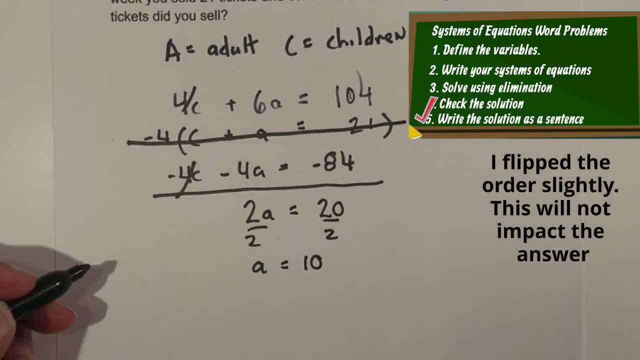 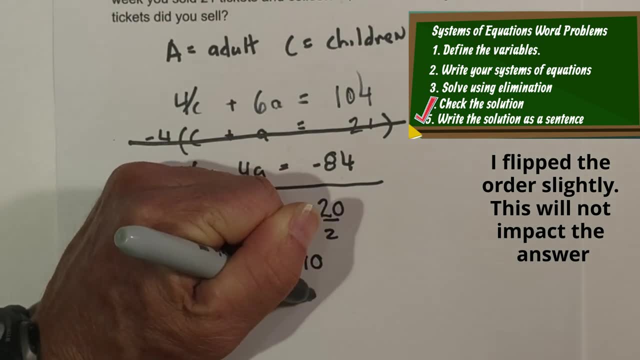 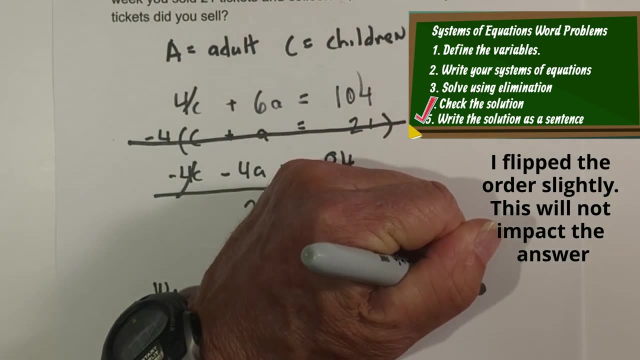 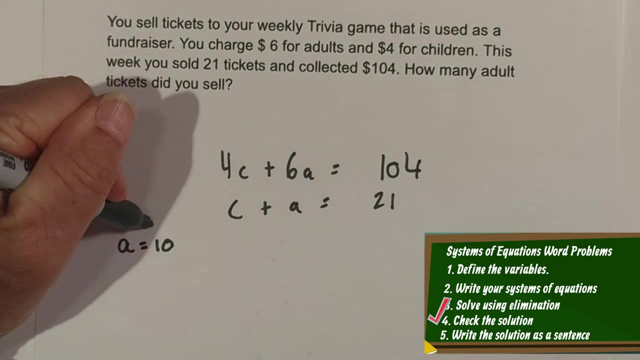 So I'm now going to write this in a sentence: We sold 10 adult tickets to Trivia. Okay, now we need to check our work. We know that adult tickets we sold 10.. So if we take 21 minus 10, that gives us 11.. 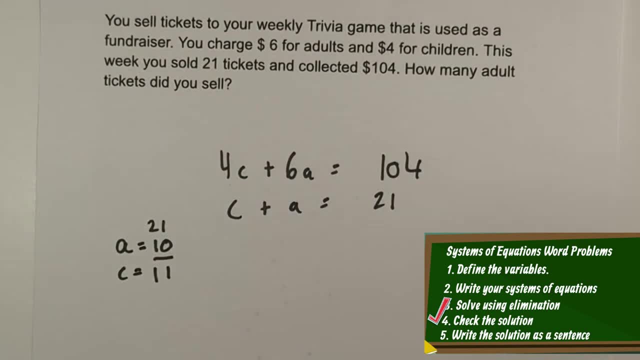 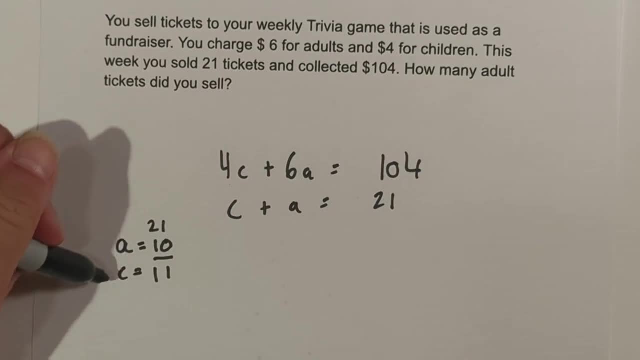 That has to be how many Children tickets we sold. So now what we need to do is plug them back into the formulas. okay, So let's start with this easy one first. We have: c is 11 and a is 10.. 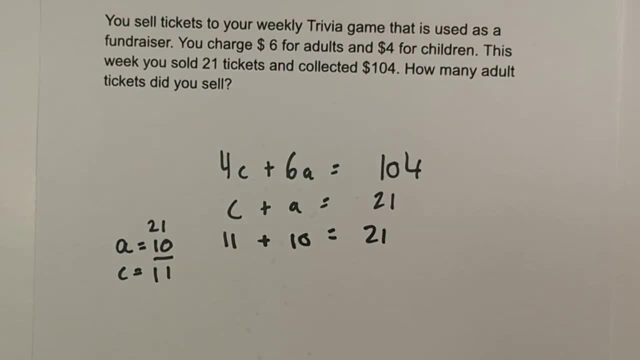 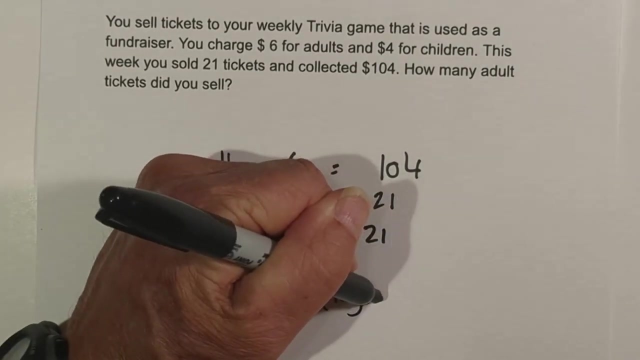 10 plus 11 is 21.. So far that checks out. So now let's try the second one. And we have 4 times c, which is 11,, plus 6 times a, which is 10.. And that needs to equal 104..